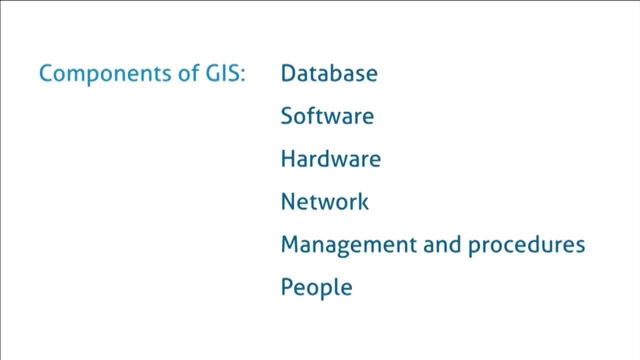 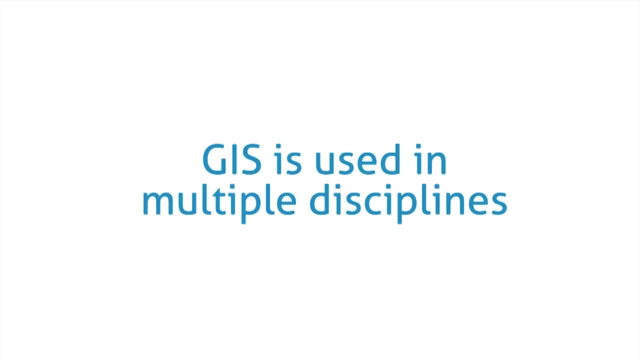 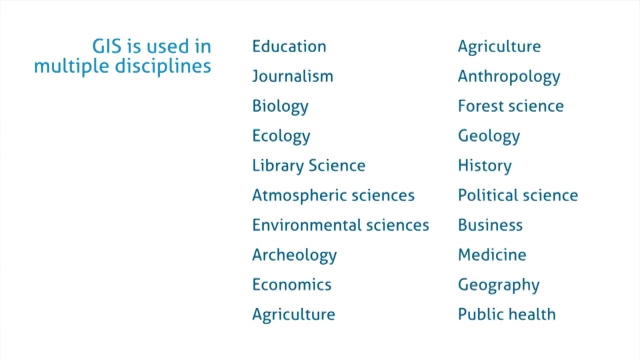 people who do the analysis. These are all the different components of GIS. So who uses GIS? GIS is used in multiple disciplines. You might find people using GIS in the fields of biology or ecology, archaeology, economics, geology, history, business, medicine, etc. So GIS has a wide 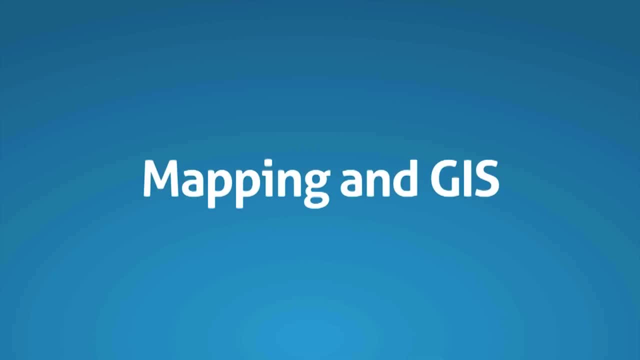 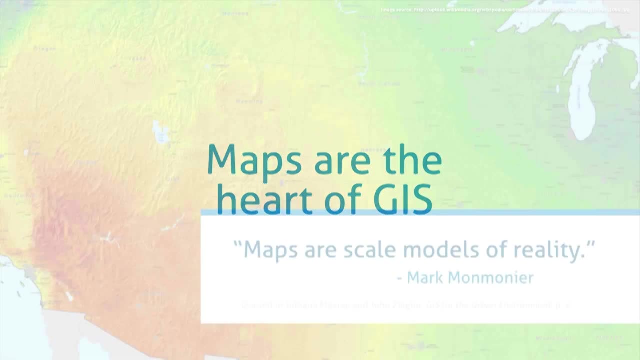 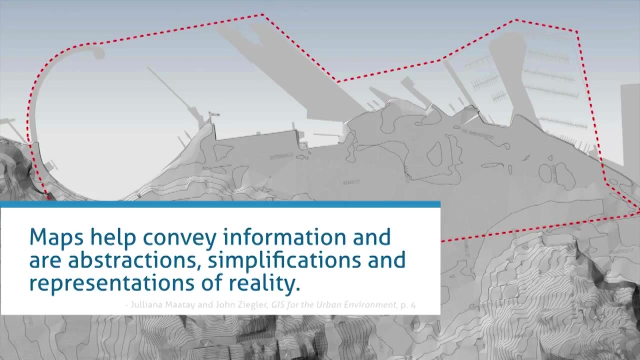 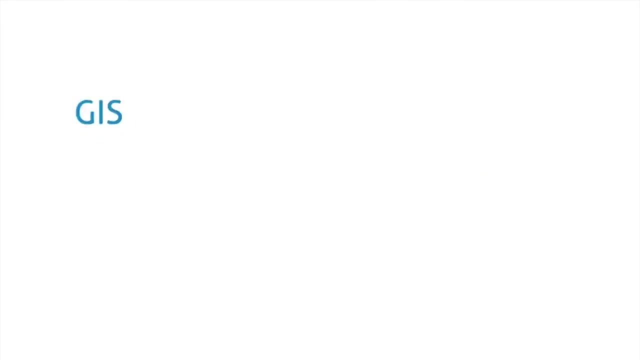 range of applications in multiple fields. Let's talk about maps in GIS. Maps are the heart of GIS. GIS is all about spatial information. Maps are scale models of reality. Maps help convey information and they are abstractions or simplifications of the real world. But GIS is more than just maps, because it's not. 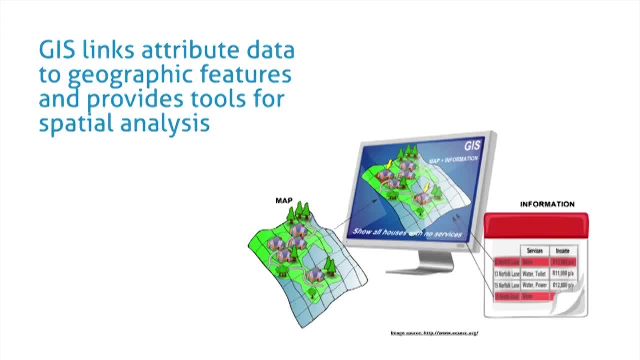 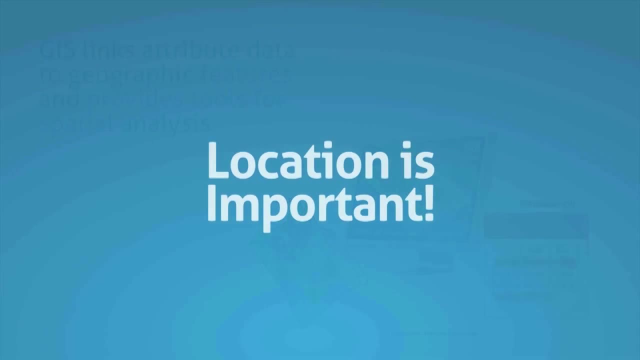 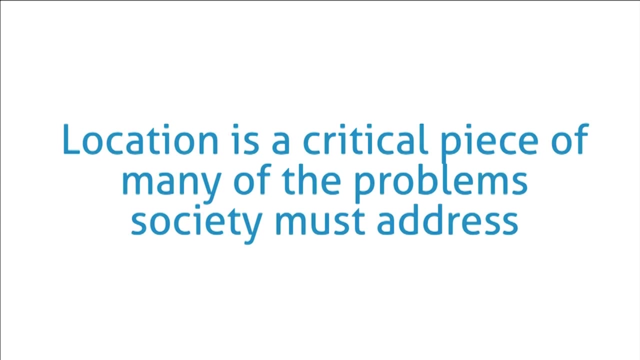 just a 2D flat map. It includes the attribute data to geographic features and allows the tools for spatial analysis. So it's not just maps. It includes the database and the ability to do the more sophisticated analysis behind it. In many disciplines, location is a critical piece of information that we have to understand when we're 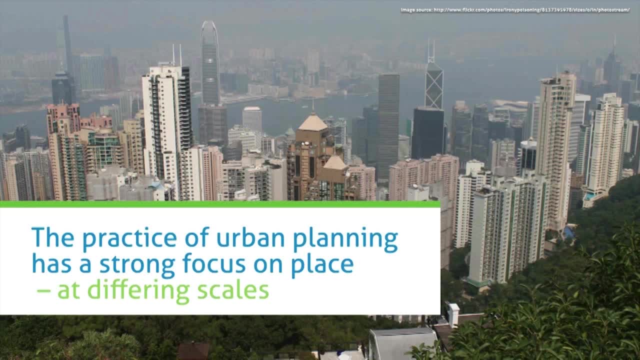 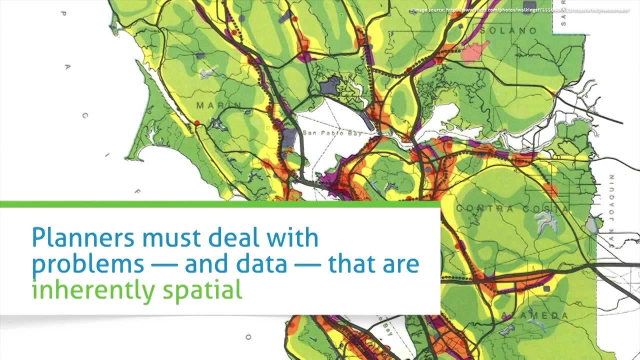 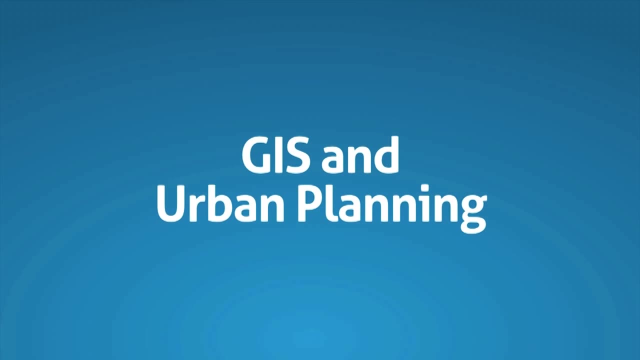 trying to think about the problems that society must address. For example, in urban planning, there's a very strong focus on place and understanding place. at different scales, Planners have to deal with problems and data that are inherently spatial in nature, So GIS is an incredibly helpful tool in the 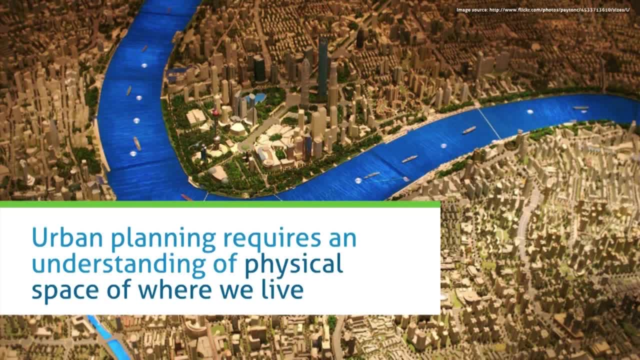 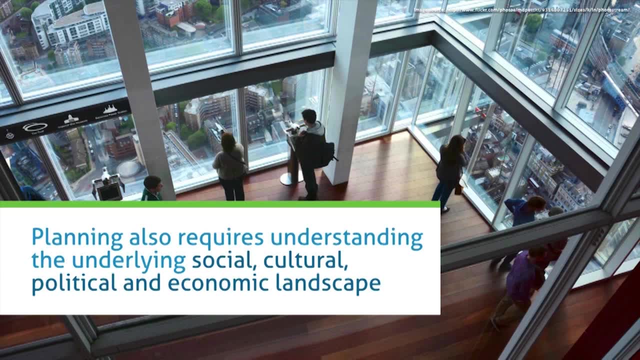 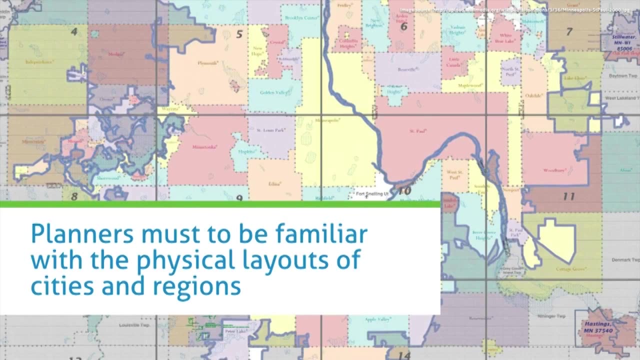 field of urban planning. Urban planning requires not only an understanding of the physical space where we live, but also an understanding of those underlying social, cultural, political and economic landscapes. So GIS helps inform planning decisions, because planners must be familiar with the physical layout of cities. 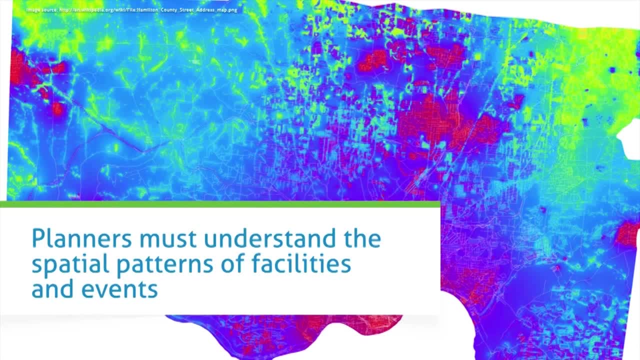 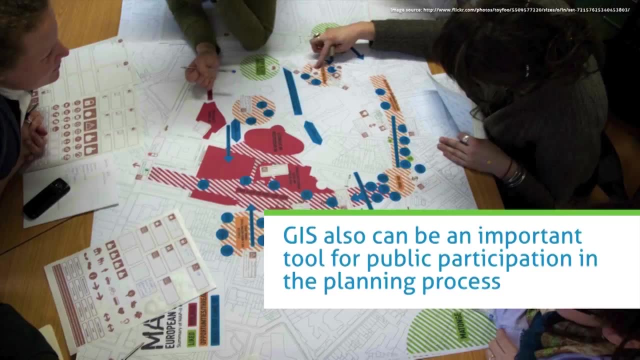 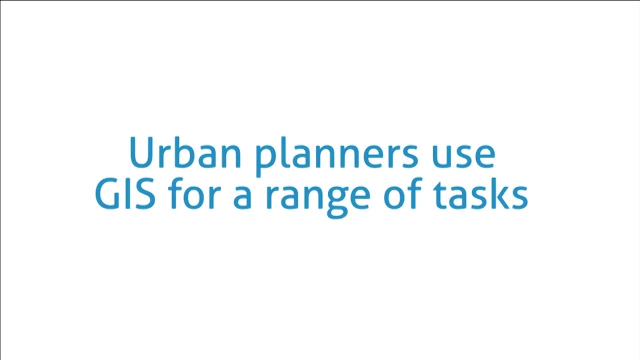 and regions, and they must understand the spatial patterns of facilities and events. GIS is an important tool for the public participation process, for helping explain spatial problems to the general public. Urban planners also use GIS for a wide range of tasks. So for all the things that planners do, for things like